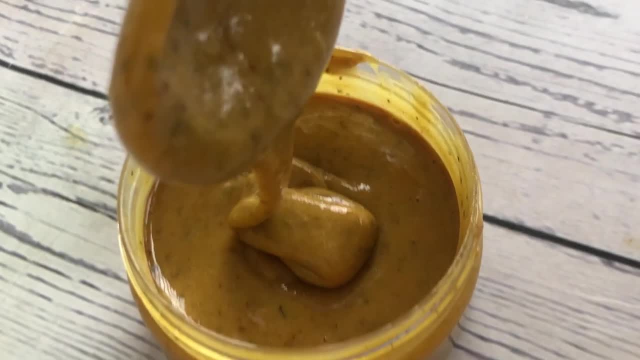 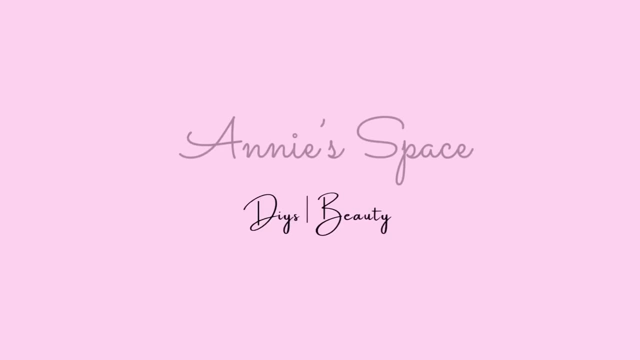 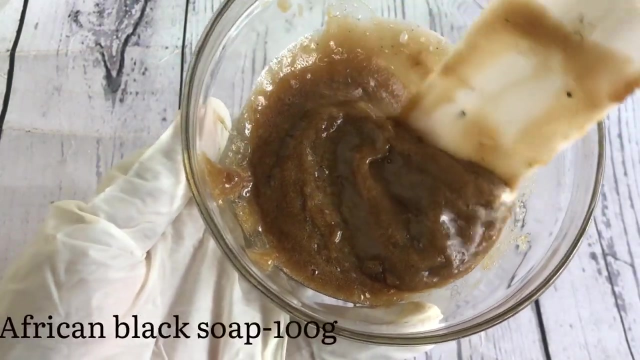 Hello beautiful people. in this video I'm going to show you how to make a very simple and mild black soap for kids. So sit back, relax and learn To make our black soap for kids. of course, we need our African black soap. This is the black 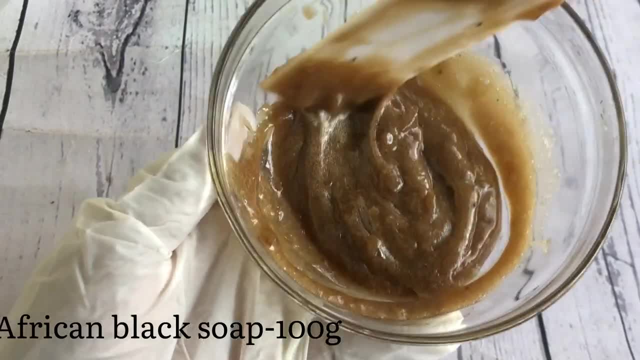 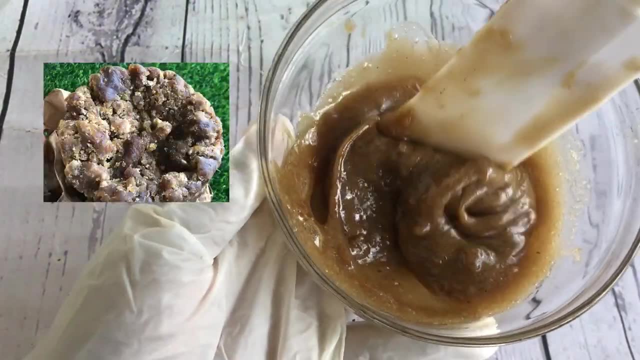 soap I melted in the video before this. You can check the link in the description box for that video to learn how to melt your black soap like this. But if you don't want to melt your black soap, you can also use the raw African black soap. that is also perfect, Because this black 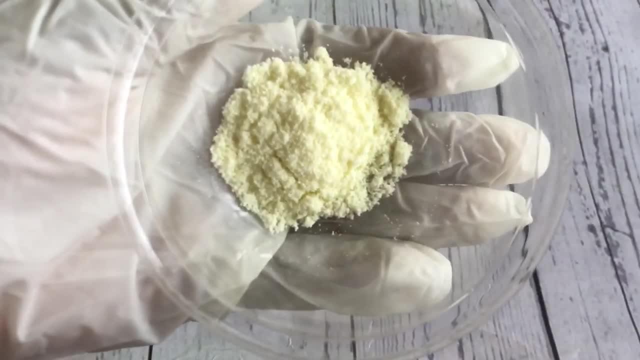 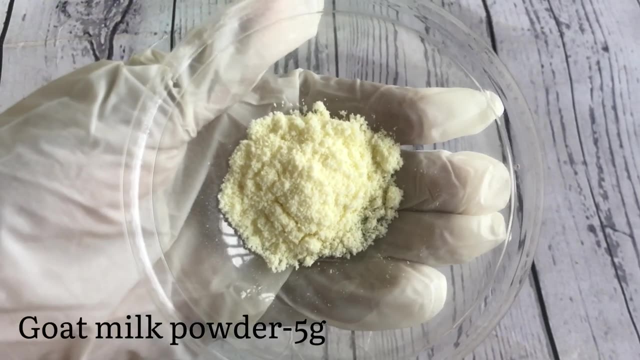 soap is for kids, we have to be very careful of the ingredients. we add Nothing too harsh, just mild ingredients. And the first one we are adding is goat milk powder. Goat milk powder is an emollient. It will help to soften the skin and also moisturize the skin of the kids. Goat milk. 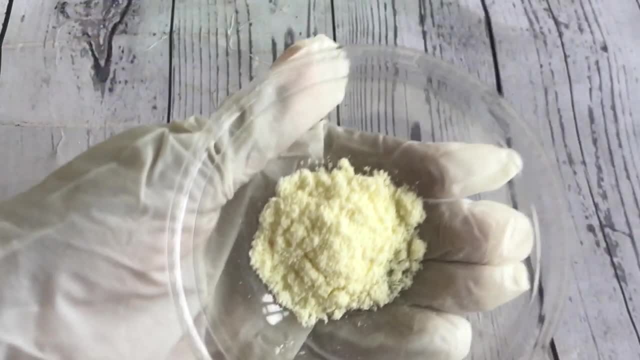 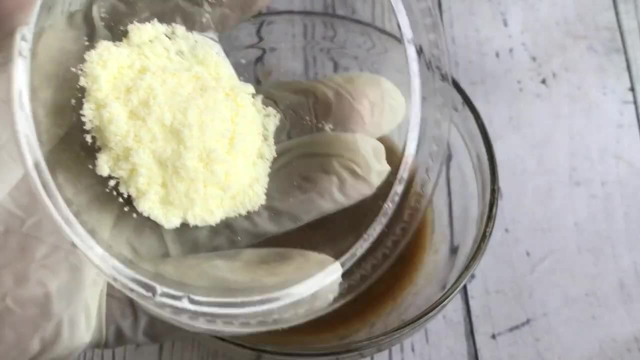 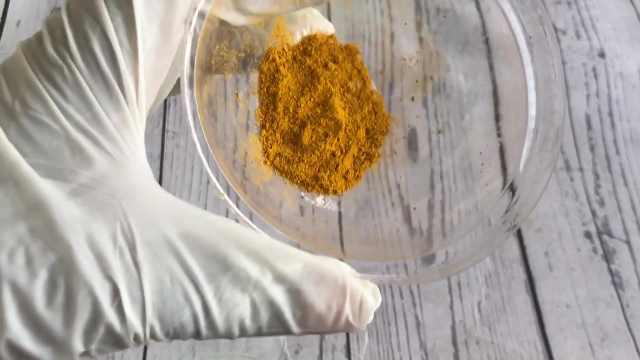 powder has a lot of benefits for the skin and it's really, really great for children's skin. The next powder we are using is turmeric powder, and we are using turmeric powder for its anti-fungal and antibacterial properties. It will help protect the kid's skin from infections, rashes and so on. 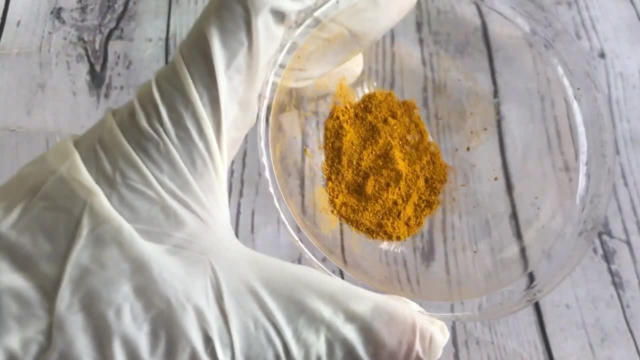 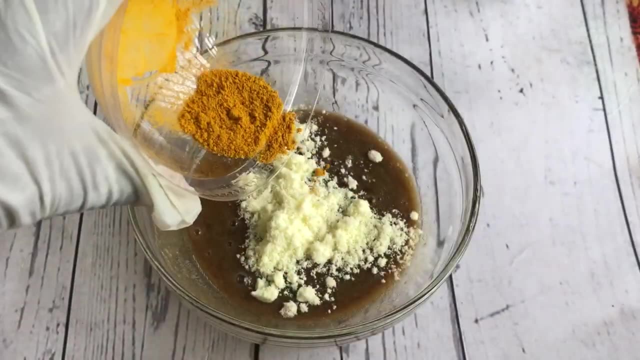 So now we're going to add the turmeric powder into the black soap as well. The full recipe with the accurate measurements will be in the description box below. So there you have it, the black soap powder. Now it's time to add the turmeric powder to your milk powder. So I'm going. 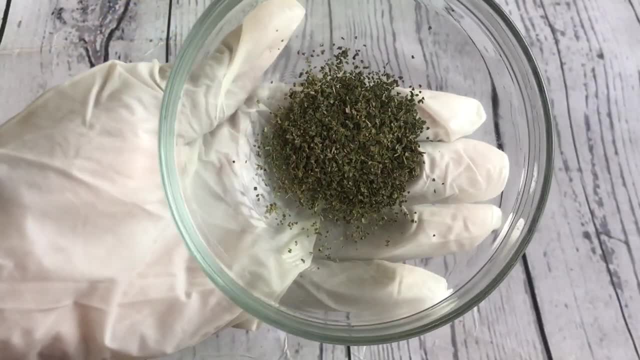 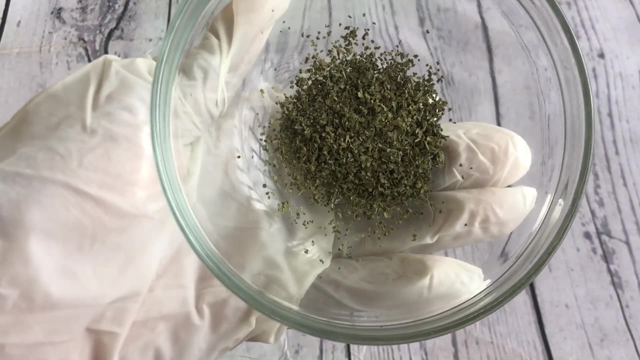 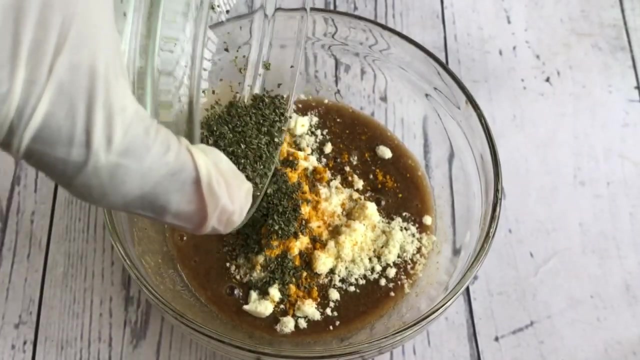 description box. check it out after watching. we'll also be adding in neem powder. neem powder is also antibacterial and antifungal. kids tend to have really sensitive skin so we need as much protection as possible from bacteria. so also we'll add the neem powder into the black soup. 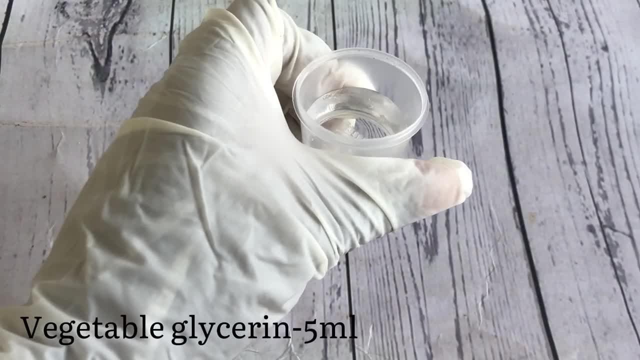 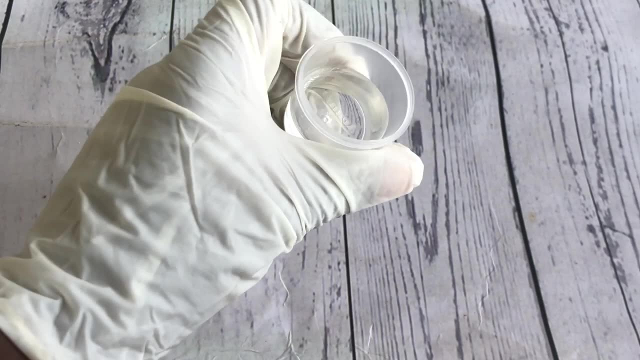 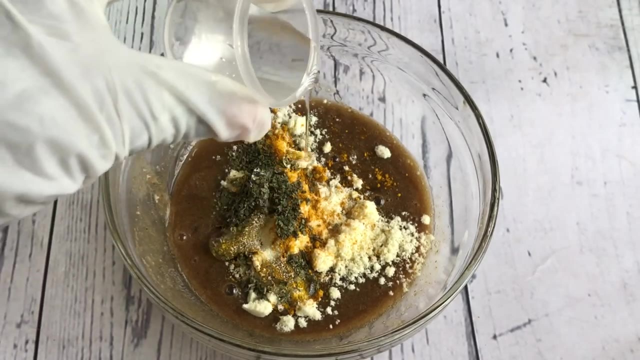 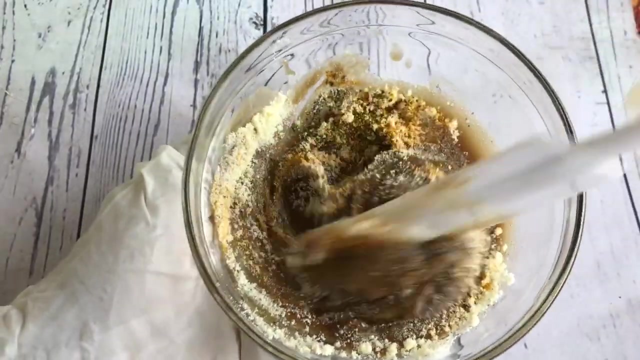 next we have vegetable glycerin. vegetable glycerin is an emulsant. it helps to draw in moisture to the skin, so we also need our kids skin to be very moisturized and hydrated, so we'll add this also into the black soup. now it's time to combine the ingredients together. we're going to mix until all. 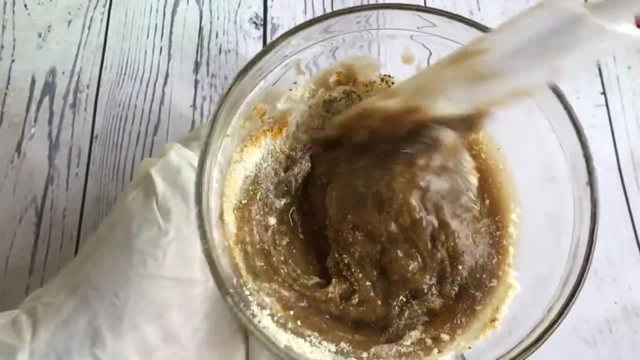 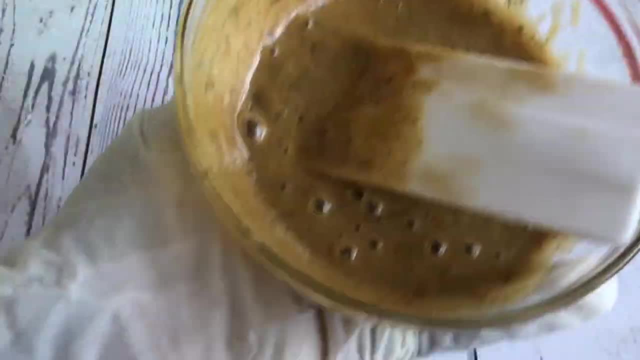 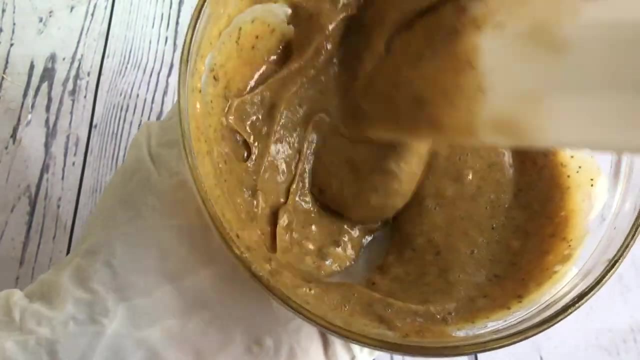 the ingredients are well and properly combined, and this is the benefit of melting the black soup first. it's just easier to combine the ingredients together, unlike when the black soup is still in the solid form state. once you're sure everything is well combined, we can move to the next set of ingredients. 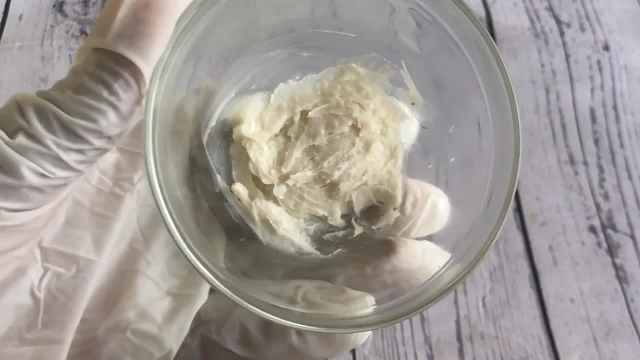 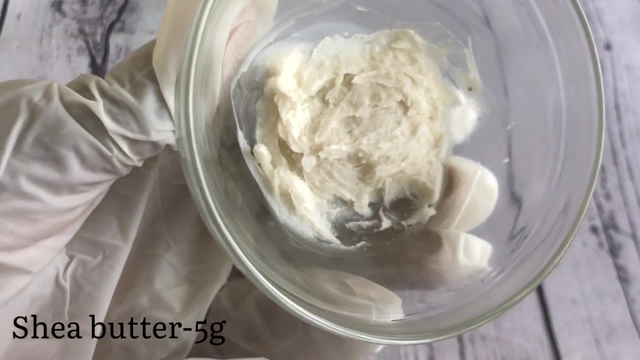 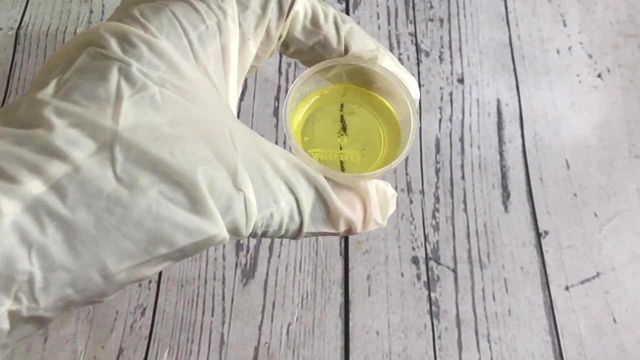 now we move to the oil-based ingredients. first here i have my shea butter. shea butter is a moisturizer. it helps to moisturize the skin, and we need the kids skin to be well moisturized, so of course, shea butter is great. next i have my jojoba oil. this is one of the best carrier oils. 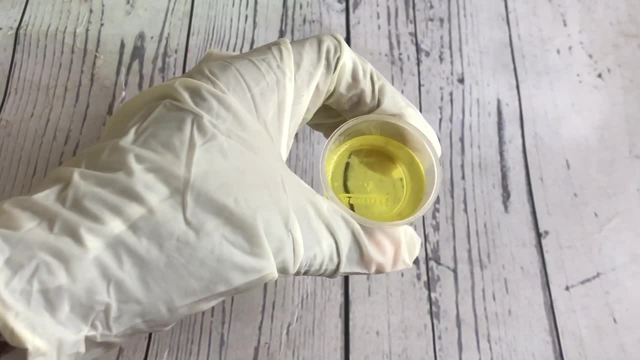 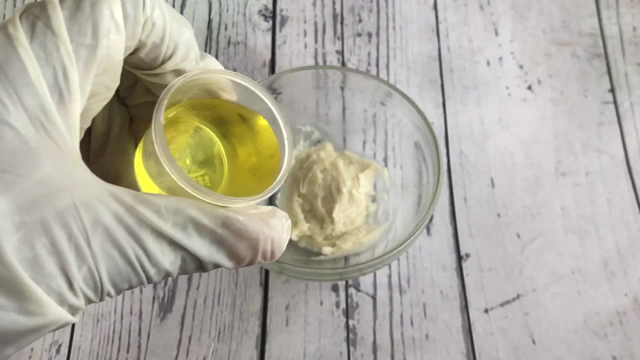 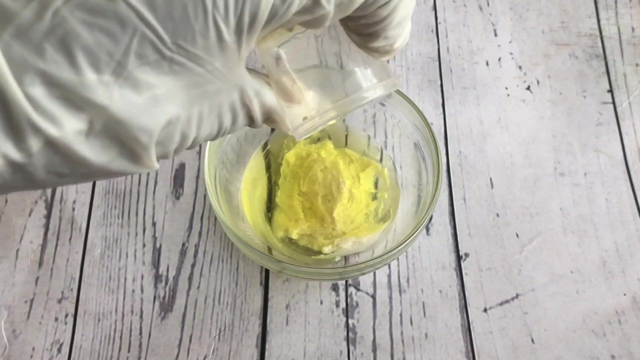 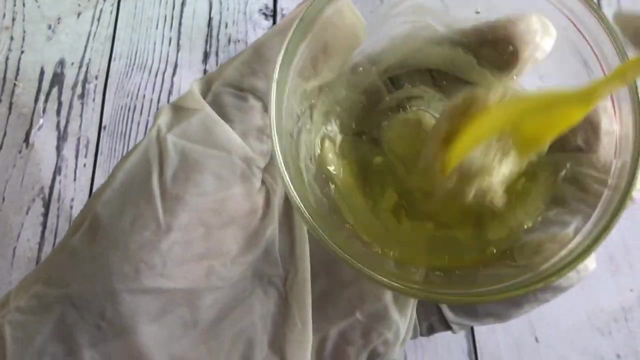 for kids. you can also use coconut oil or calendula oil. both are also great for kids skin. so we'll be using jojoba oil and i'm going to add the oil into the shea butter now. now i'm going to mix the both of them together so that the shea butter can be properly dissolved. 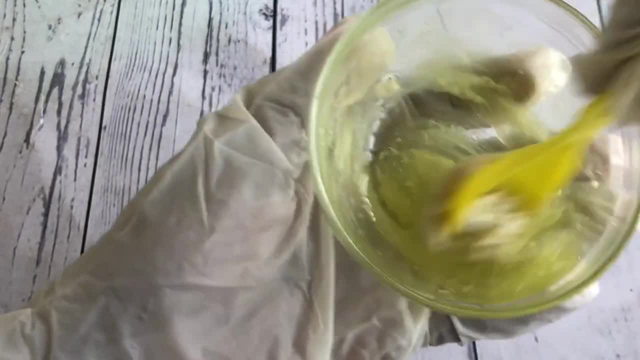 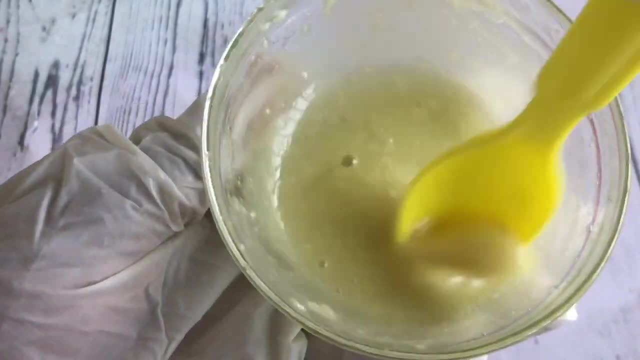 because you can't add a very solid shea butter into the soup. you can also use a double boiling method to melt the shea butter, but i'm going to use a double boiling method to melt the shea butter, but i'm not using that right now. i'll just mix until everything is well dissolved, as you can see. 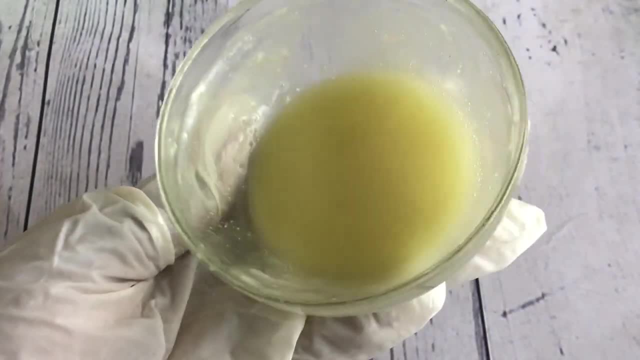 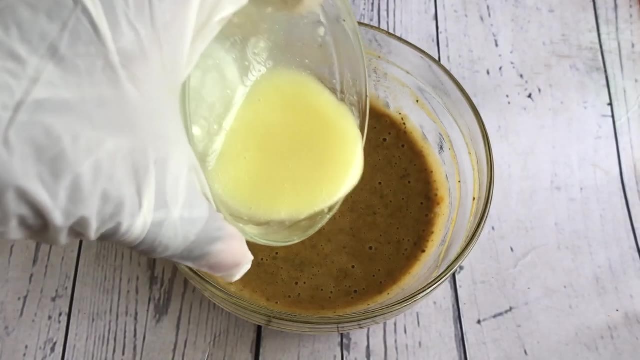 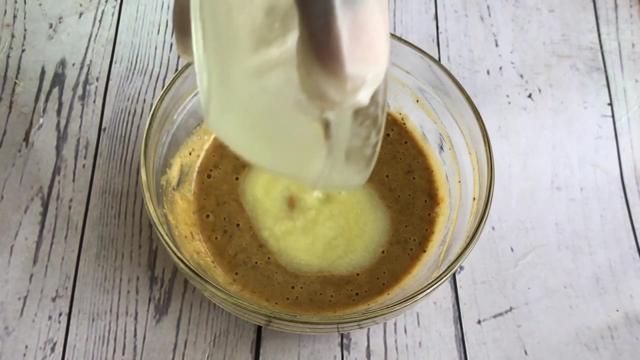 it's already dissolving. now that our shea butter is properly dissolved in the jojoba oil, we're going to add it into the black soup as well. in place of shea butter, you can also use mango butter, cocoa butter or any other butter. all of them are perfect for kids. so now, after adding the shea butter, we're 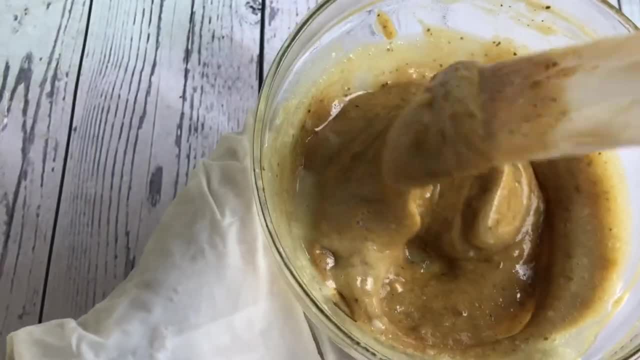 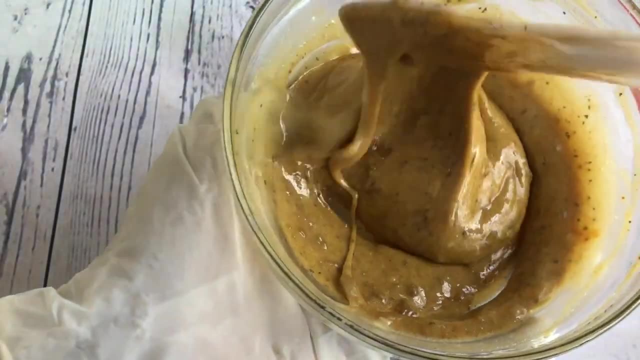 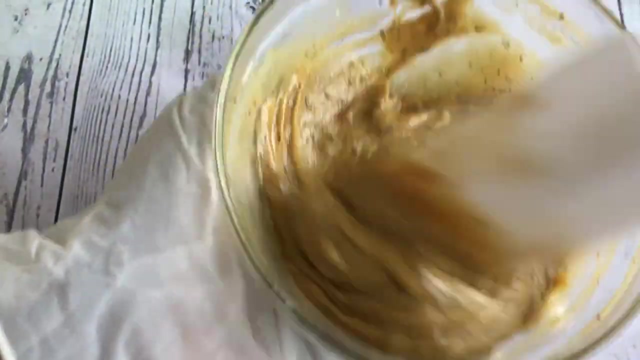 going to mix it in until it's properly dissolved, and then we're going to add the jojoba oil to the mix with the rest of the black soup. this is a very little quantity of black soap and, moreover, i did not add any form of water into this black soup, so adding a preservative is not so compulsory, but i'm 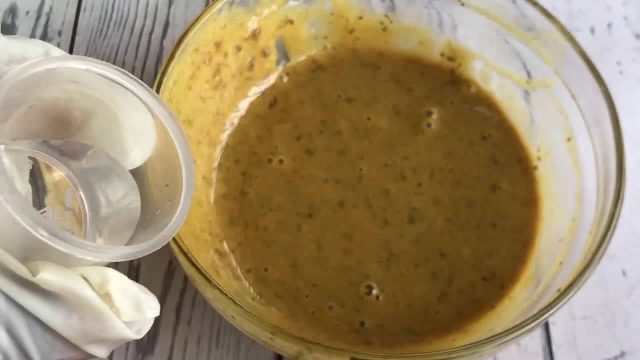 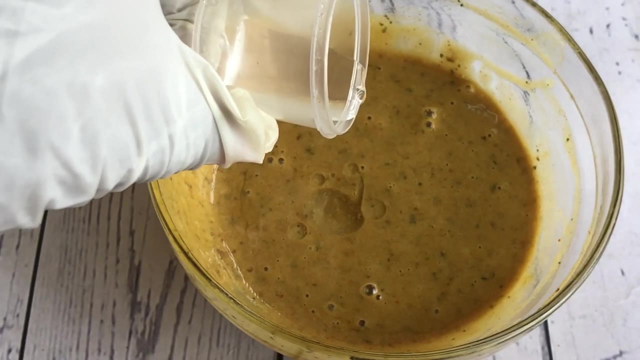 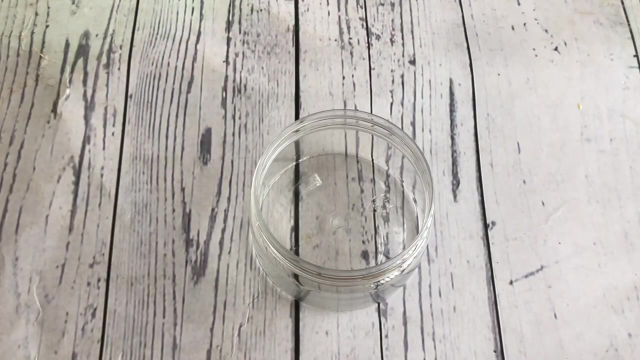 going to add preservative anyways, you can decide to skip this if you're making very little batch and you are sure that you will exhaust it in no time. once more, we're going to give it a very good mix to make sure that the preservative goes all around the black soup, and now we're going to put it in our jar if you don't melt your black.